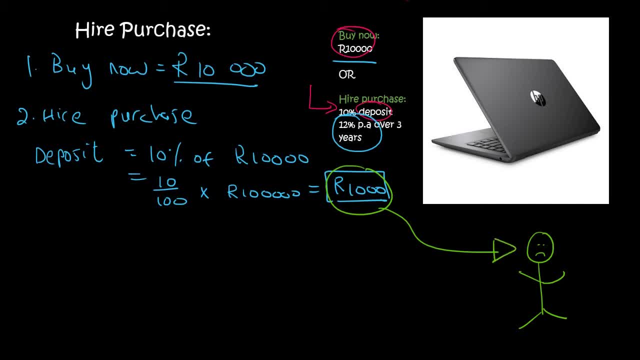 because you haven't given him the full amount. So you've given him 1,000 Rand. So how much do you still owe on the laptop? Well, that laptop is 10,000 Rand And if you minus the 1,000 Rand, you still owe this guy. 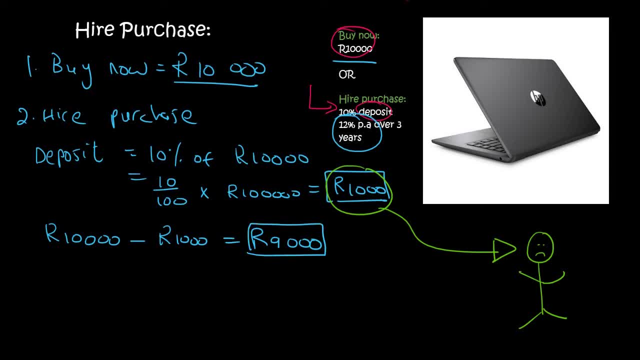 9,000 Rand. So he's a little bit upset with you because you still owe him 9,000 Rand. So what he's going to do is he is going to take this 9,000 Rand and he's going to add interest. 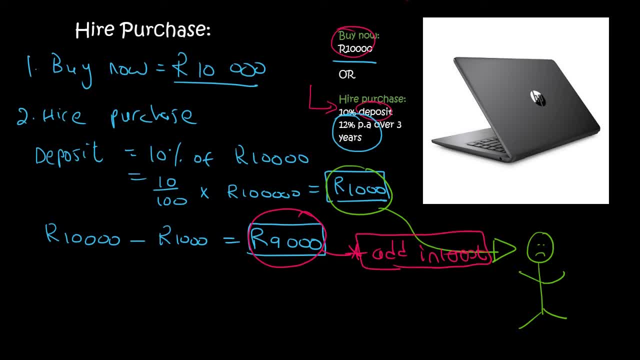 Okay, And he's going to add money on to that so that you end up having to pay him a little bit more. That's fair. You're not giving him the full amount, So he's letting you take the laptop for 1,000 Rand, but he wants you to pay the 9,000 Rand back. 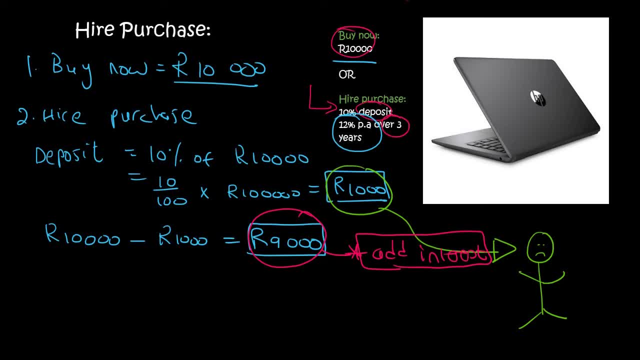 But you're also going to pay a little bit more and you're going to do it over three years. So he's going to add interest on and he's going to do that using simple interest. Remember, we've learned about simple and compound. 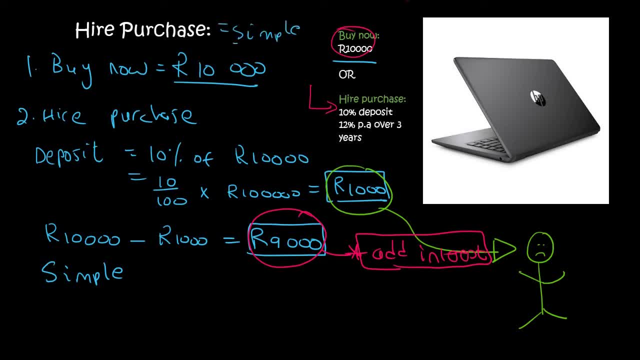 Higher purchase is always simple, Simple. please remember that. higher purchase simple, higher purchase simple, higher purchase, simple. So we use the simple interest formula and we're not going to use 10,000 as the starting amount This person is only going to. they're only upset because of the 9,000 Rand that you haven't paid. 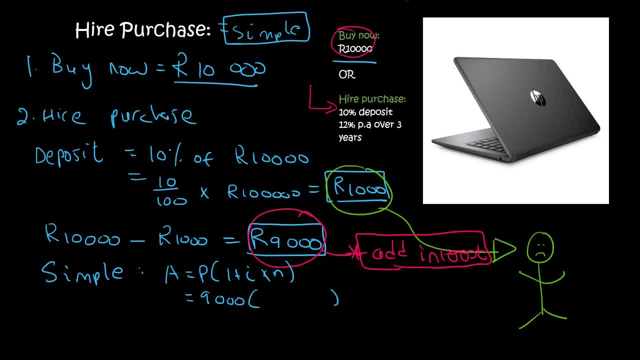 So they're going to take that 9,000 Rand and they're going to add interest. Now in the advert they said 12% per year, so that's 12 over 100 or 0.12.. And then that's going to be over a three-year period. 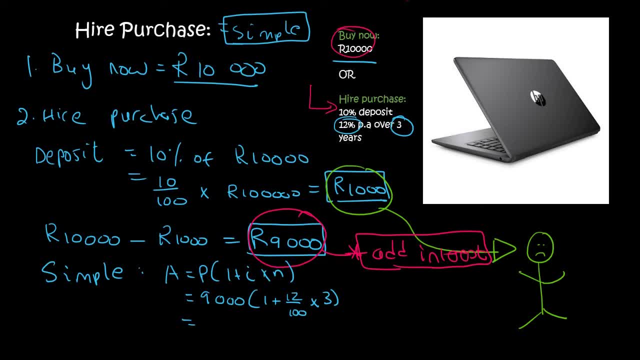 And so let's see what that 9,000 Rand is going to turn into. Wow, 12,240 Rand. So imagine this: guys, You've already paid 1,000 Rand. Then the man takes that 9,000 Rand that you still owe him and he says: hey, by the way, I'm turning that 9,000 Rand into 12,240 Rand.